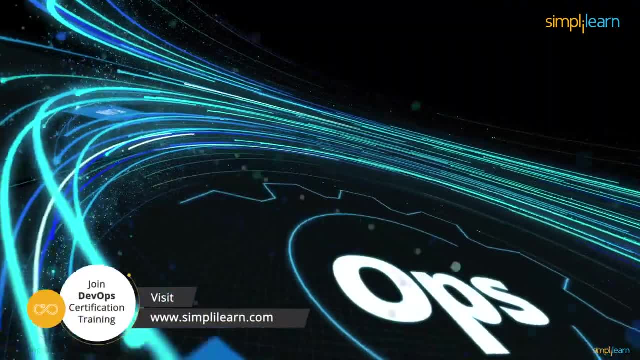 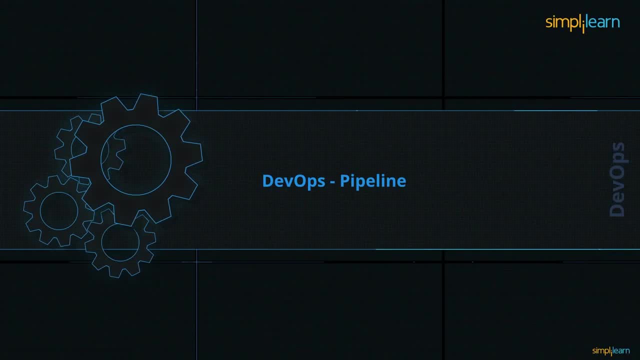 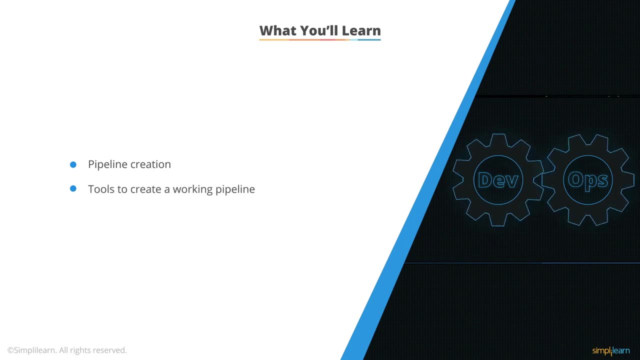 Hello and welcome to DevOps Pipeline Setup and Creation using Various Tools- Introduction Session. We will look at what a pipeline is, what is pipeline creation and what are the various tools available on the market to create a working pipeline in a DevOps project. 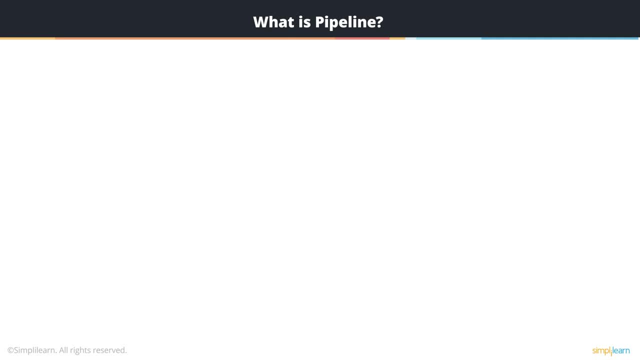 So what exactly is a pipeline? A DevOps pipeline is essentially your setup in a software project that helps to deliver continuous integration, continuous deployment and eventually finally leading to continuous delivery of your software project. We will discuss continuous integration, continuous deployment and what exactly do we mean by continuous delivery. 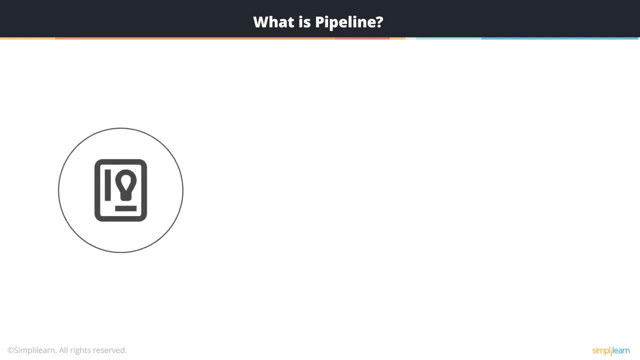 in more detail here. So the idea behind creating a pipeline is to be able to create a repeatable and reliable system and be able to continuously improve the process of software development and delivery In order to make your software delivery from concept stage to your customer faster. 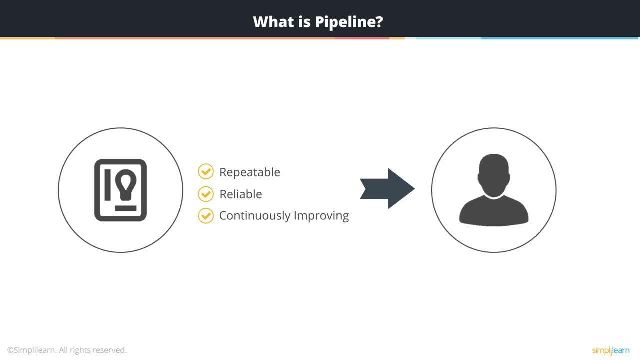 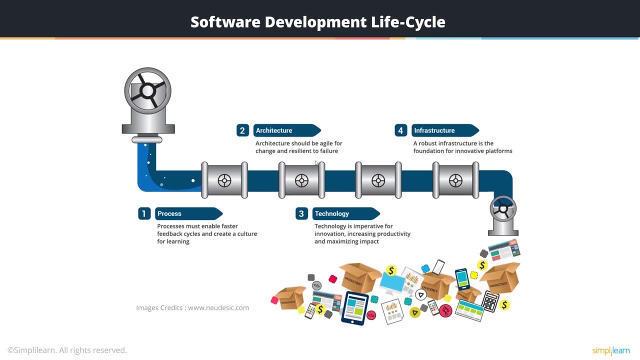 The goal here is to enable a constant flow of changes into production using an automated process by including various tools at each of the steps. So this is how our software development lifecycle pipeline typically looks. You have processes that must enable faster feedback cycles and create a culture for learning The architecture for your software development lifecycle. 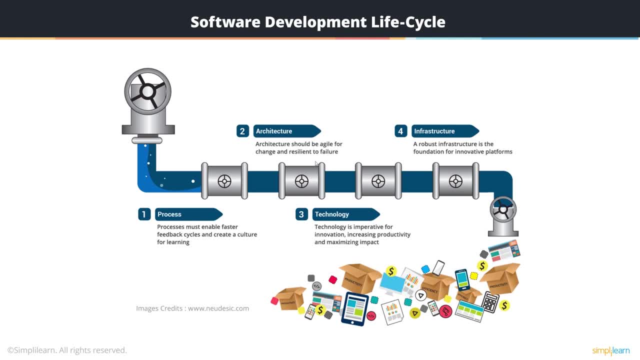 for the software that you're working on is a very important part of the process. You need to be agile for change and resilient to failure. You need to be able to take what you learn from what is failing or not working back to your process faster and make the appropriate. 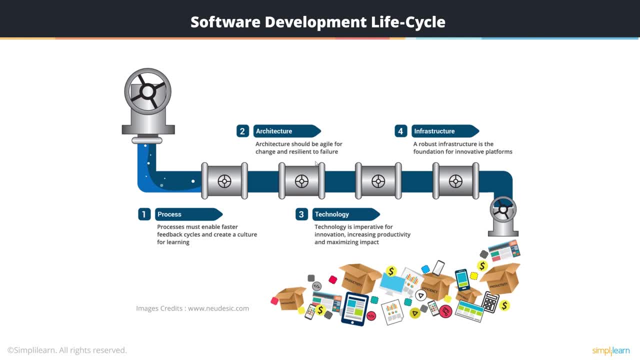 changes and continue with the pipeline. You need to have the necessary technology that enables you to implement a pipeline that helps you to increase productivity and maximize the impact of the software that you are developing. So for technology, you should have the right tools and the necessary software. 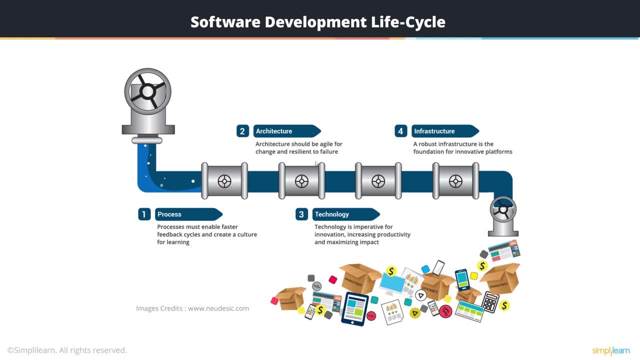 You need an appropriate, robust infrastructure, such as servers, cloud environments, virtual machines and various innovative platforms that enable creation of a pipeline, setup of a pipeline, working of a pipeline and eventually deploying the software that you are creating using a pipeline into your production environment and then on into an environment. 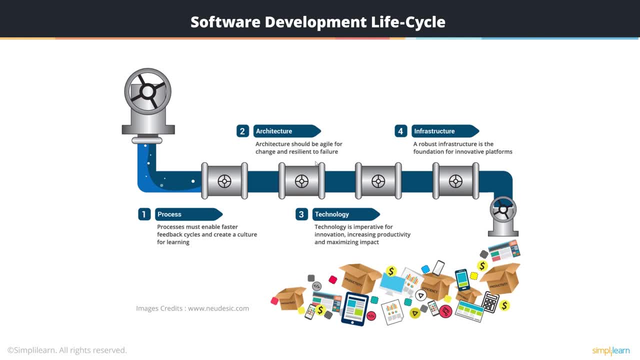 that your users can access and have permission to look at. So to begin with, you need to have the right tools and the necessary infrastructure. You need to know why you would implement mind bluan or fear MASCH. reason to have an open. 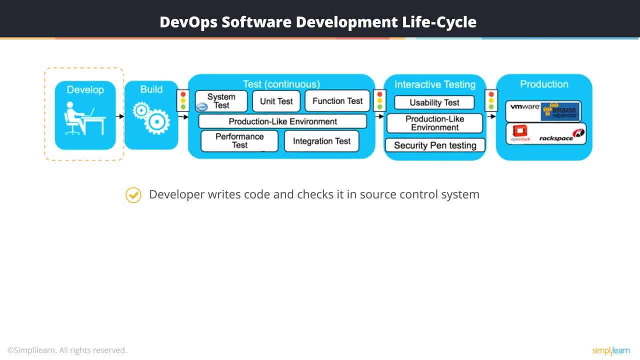 江, or to have a non-denial plan agreement with the end user Once you have an in す Kollege with the AAA Fool. Thank you, We're about to start our presentation, So we'll begin with Master Information. As you can see, you're going to provide USA Mesos with the necessary features that allow. 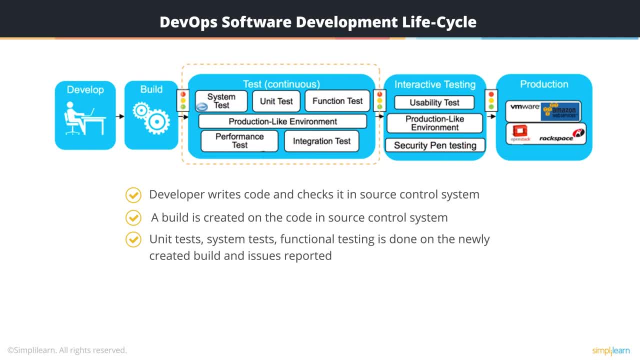 environment, UAT or staging. Then, finally, you get to do the security and penetration testing. once the build is ready for production, Then your production environment is created and set up and the final build is deployed for your end customer- These things that we just discussed. 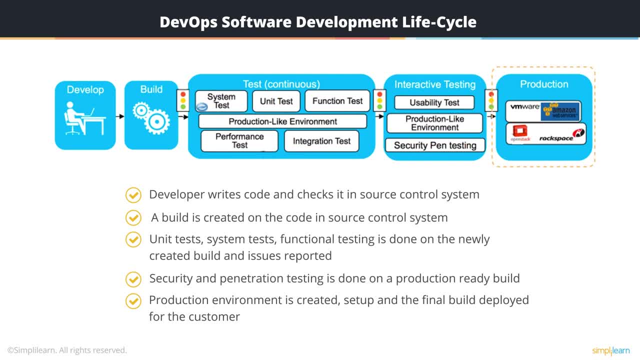 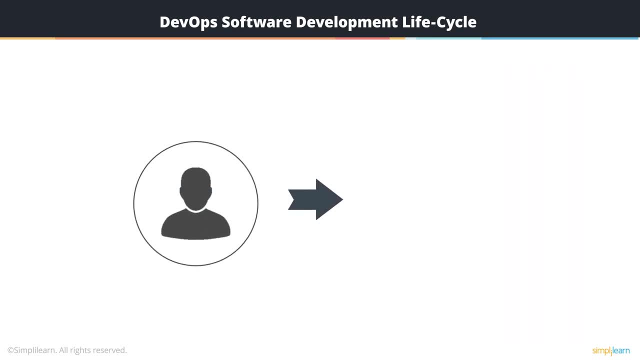 are typical steps that we follow in an SDLC lifecycle for our software development and delivery. A lot of these steps are done manually. Manual steps make these less repeatable, more error-prone and more time-consuming. Environment setups are long drawn-out processes and build. 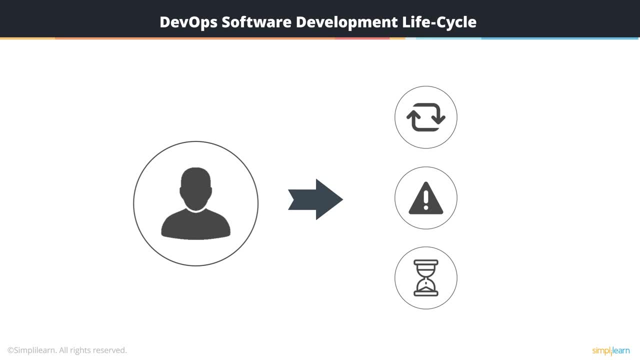 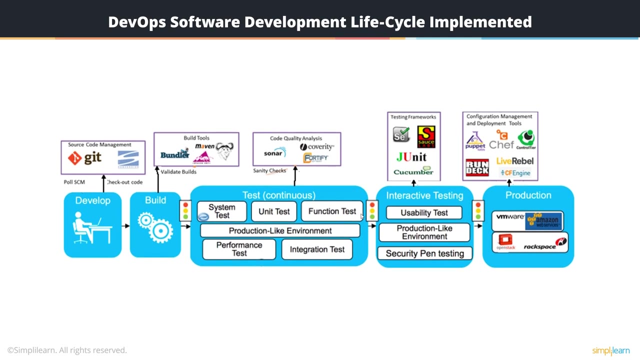 creation deployments are very time-consuming, taking up team member time throughout the entire project, And this is time that could be better utilized on other more important tasks or tasks that improve the overall quality of the deliverable or increase the functionality you're trying to deliver to your customer. Now, this is how it would look if you were to deliver all the DevOps SDLC. 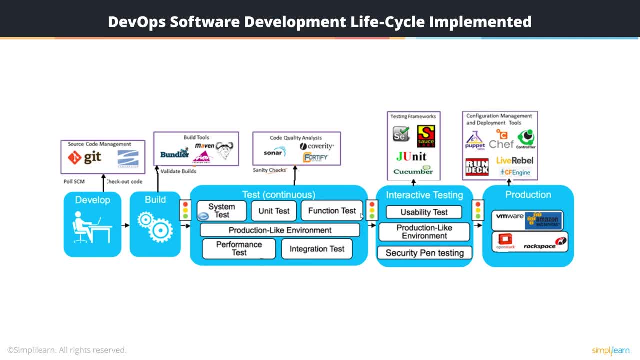 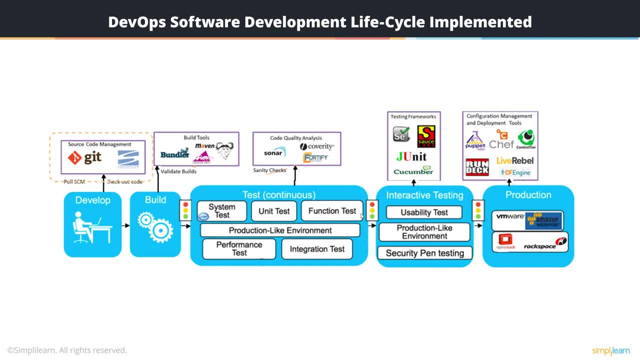 which can be continuously pulled using a continuous integration system like jenkins that can run various tools like maven or ant to create a build from the code in your source code repository. So this can all be automated Now in order to validate the build. 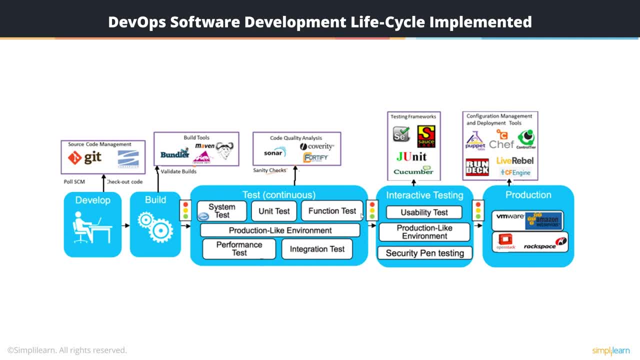 you can integrate your continuous integration server or jenkins with tools like Sonar or fortify that help you with various validation and quality checks on your builds. You can create various quality gates in Sonar that basically validates your build is good to go into production and onto your customer for consumption. You can also trigger various tests. 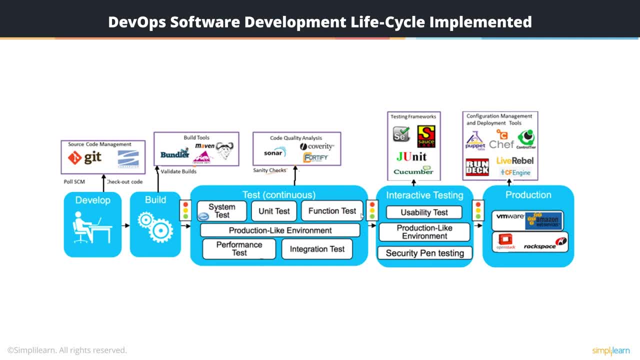 like unit tests, script tests or functional tests and all your system tests using various plugins that Jenkins provides for different test tools like JUnit, JBehave for BDD testing. You can even trigger your performance test suites and integration tests. Jenkins offers a lot of. 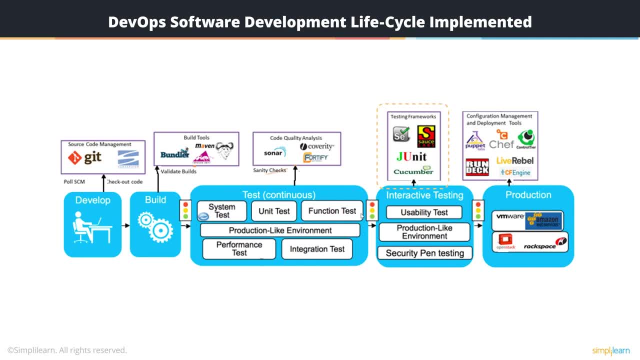 plugins for various test tools and test suites. Even Selenium and Cucumber test suites can be triggered using your Jenkins integration server. Next, in order for you to do your user acceptance testing, security, penetration testing, you can integrate your JUnit, your Selenium, your Cucumber. 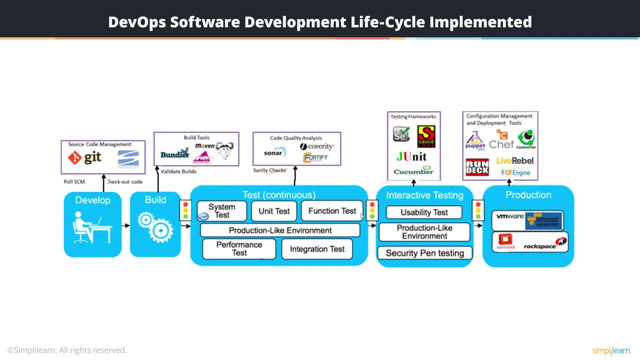 your Sauce Labs and various testing frameworks with your continuous integration server. These can automatically trigger your performance test suites and integration tests. You can also automatically trigger the scripts on various test suites that you need to run against the build. Continuous integration servers also help you configure your production environment. 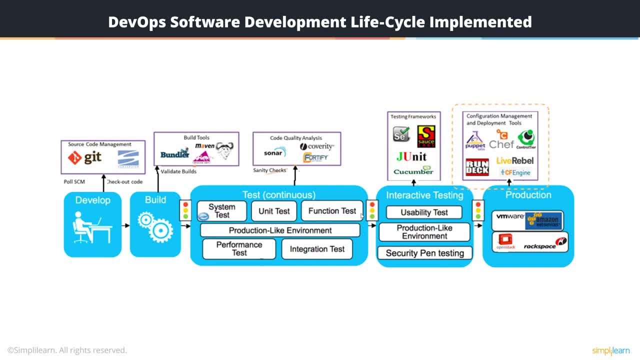 You can integrate these with tools like Puppet and Chef, which are configuration management tools, and they can help you set up your production environment, automate the creation and setup of your production environment and, finally, do your build deployment on the environment. Now, this could be a VMware environment. It could be an Amazon AWS cloud environment. 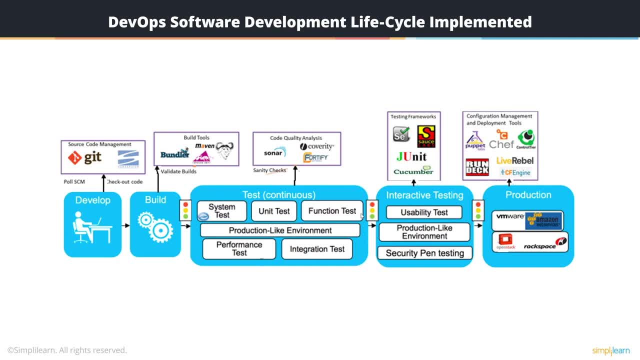 It could be a Rackspace or Open Stock. So, looking at this diagram, we have essentially converted all the manual steps from deployment to build, build to testing, test to UAT and finally to your production deployment using various tools. So essentially, we've created a software. 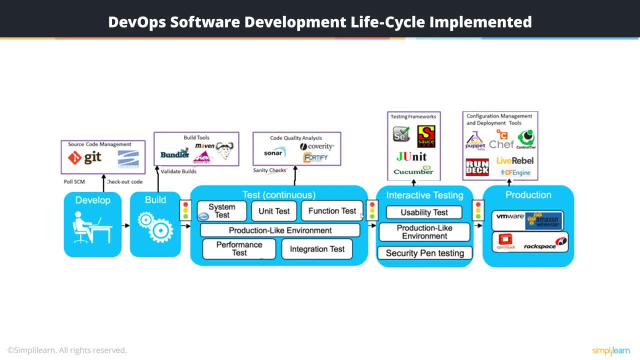 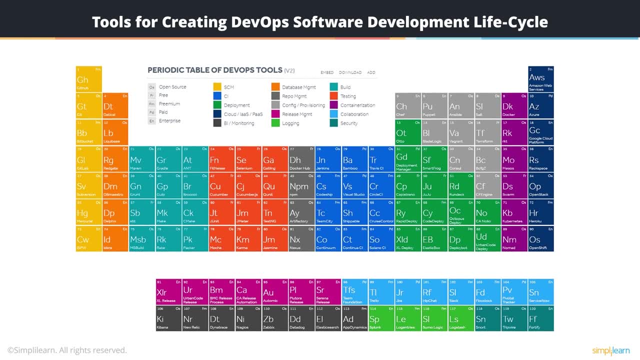 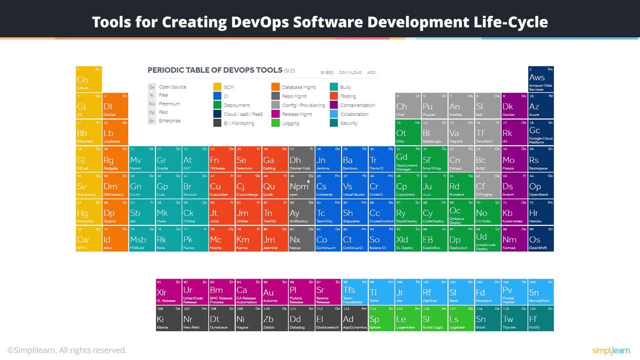 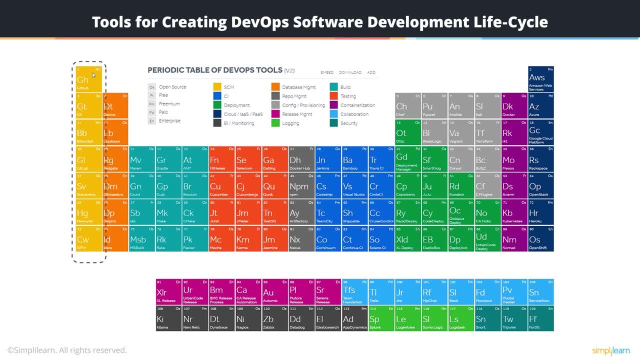 phases of your project. Here you see the various source control repositories. Next you see various databases and then you see a whole bunch of build tools. Here you have your Jenkins and Bamboo and Travis. These are your continuous integration servers. These are various deployment tools. These are various configuration management tools.